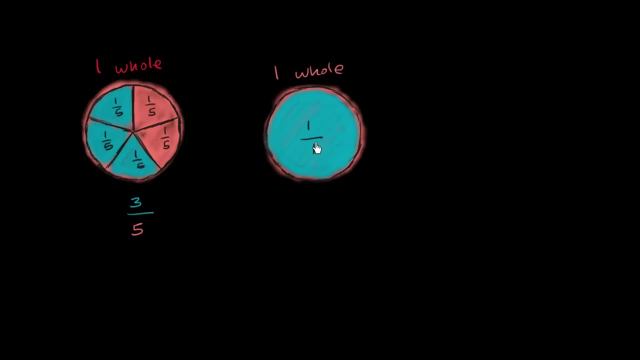 and I have shaded in exactly one of those, one equal section. I've shaded in the whole thing. Or I could say that one-oneth, which you'll never hear someone actually say, is shaded in, Or I could say that the whole thing is shaded in. 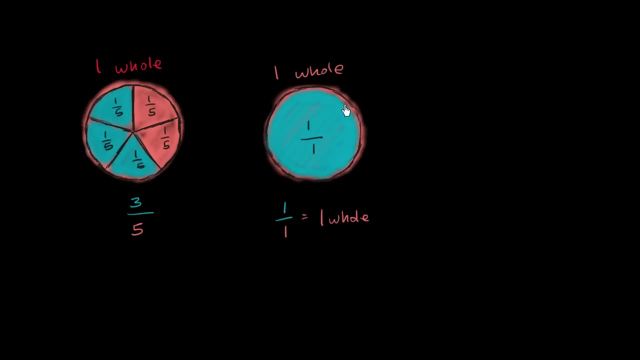 So this is equal to one hole, So that's a hole. That's interesting And I want you to keep in mind, remember: look, we have three. We literally have one, two, three and four. One, two, three, fifths. 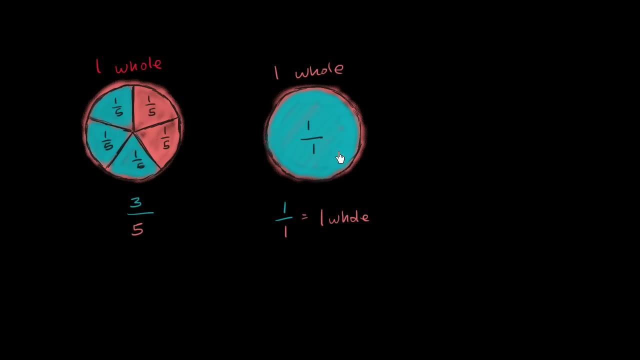 And we literally call that three fifths. Now this is one hole. Now what happens if we were to do this multiple times? So if we were to? let me copy and paste that. So now I have another one hole, and then another one hole. 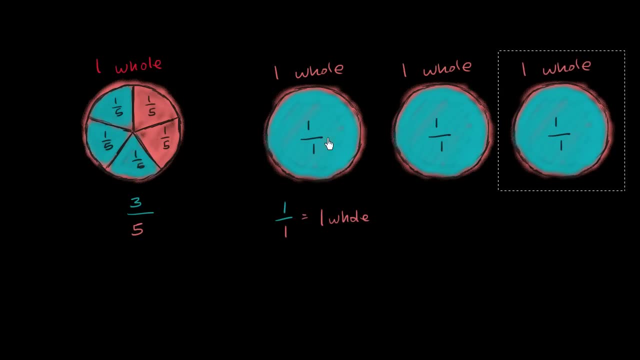 right over here. So now, in total, how many holes do I have? Well, I have three, One, two, three holes. So I could say, and I've actually shaded in three holes, So this one right over here is equal to let. 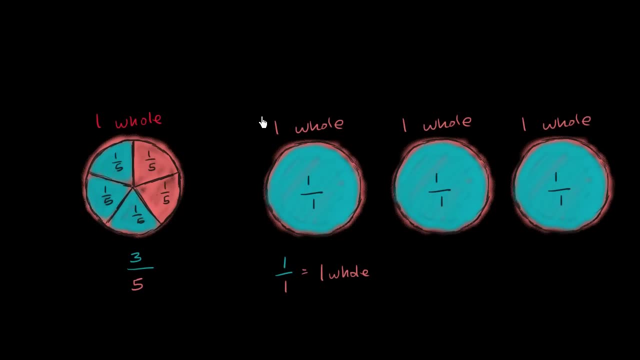 me make sure I label it right. this right over here is equal to: if I were to take the combination, this is equal to three holes. Or if I were to think of it in terms of numbers, just a number line. this is literally. 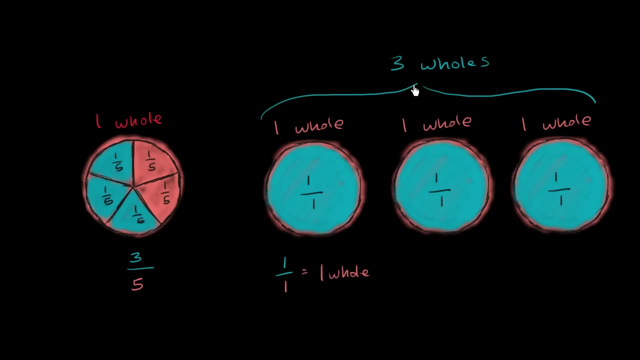 this would represent the number three, But what's another way I could represent it? Notice, when I took one fifth, another one fifth and another one fifth, I could call that three fifths. So now, if I take one, one, one, three, one fifths, then that's. 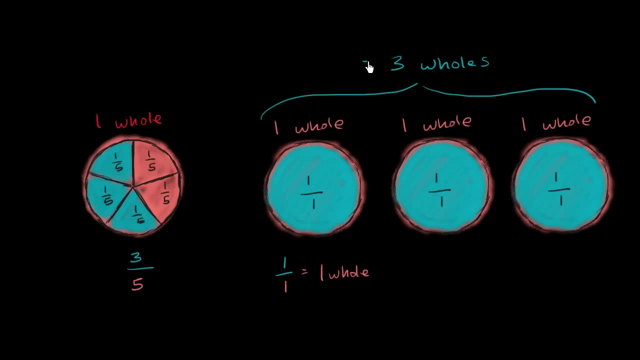 1-th, another 1-1-th and another 1-1-th. well, I should be able to call this 3 1-ths or 3 1-ths, or however you want to call it. 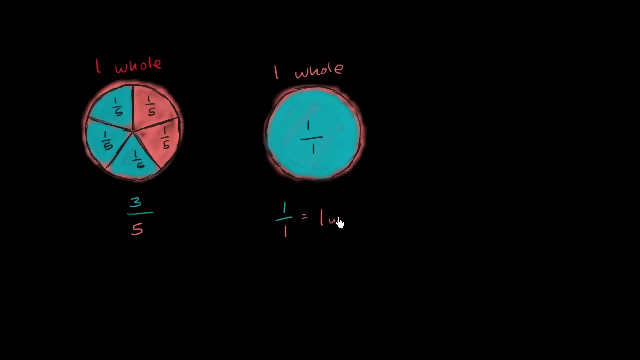 Or I could say that the whole thing is shaded in, So this is equal to one hole, So that's a hole. That's interesting And I want you to keep in mind, remember, look, we have three, We literally have one. 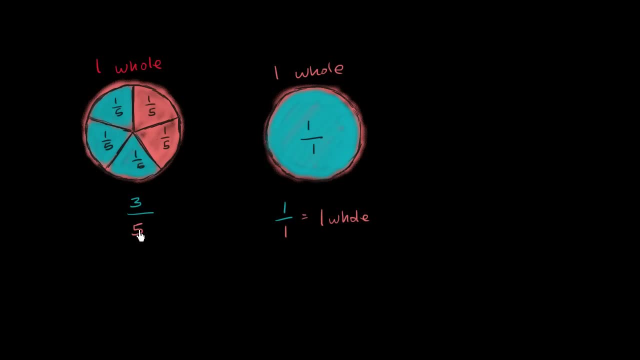 Two, Three, fifths, And we literally call that three fifths. Now, this is one hole. Now, what happens if we were to do this multiple times? So if we were to? let me copy and paste that. So now I have another one hole, and then another one hole. 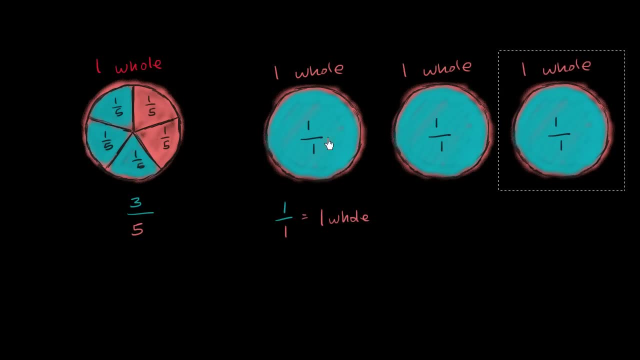 right over here. So now, in total, how many holes do I have? Well, I have three, One, two, three holes. So I could say, and I've actually shaded in three holes, So this one right over here is equal to, let me make sure. 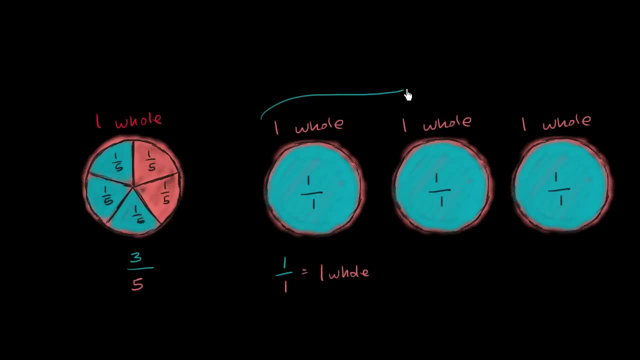 I label it right. This right over here is equal to: if I were to take the combination, this is equal to three holes. Or if I were to think of it in terms of numbers, just the number line, this is literally. this would represent the number three. 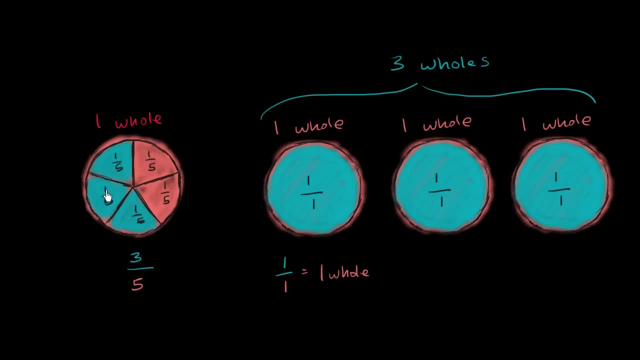 But what's another way I could represent it? Notice, when I took one fifth, another one fifth and another one fifth, I could call that three fifths. So now, if I take one one, one, Another one one and another one one. 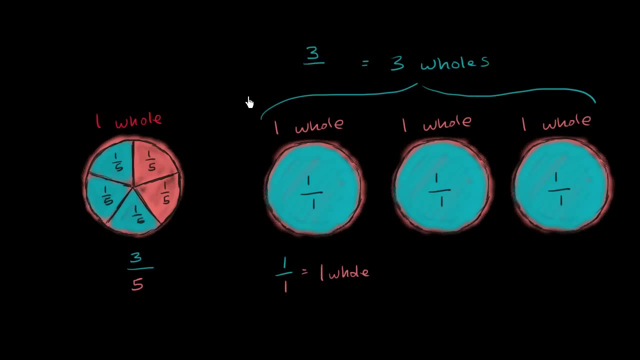 Well, I should be able to call this three once or three firsts, or however you want to call it. So I could call this three firsts. So this is interesting. Now we're seeing where the top number on a fraction is larger than the bottom one. 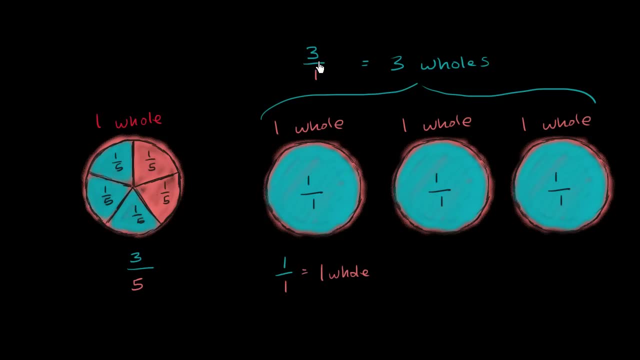 But another way of thinking about this fraction symbol is that it's division. So you could view this as three divided by one is equal to three. Or you could say, well like one over one is a whole, and I now have three of them. 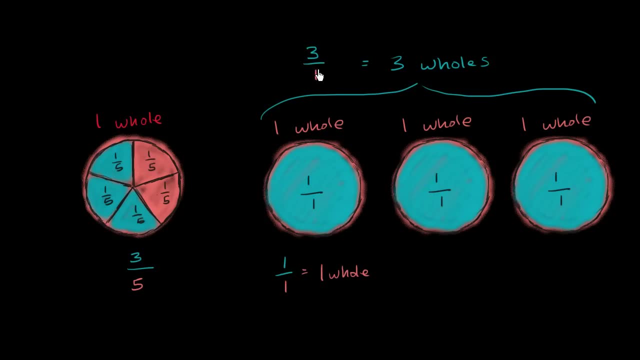 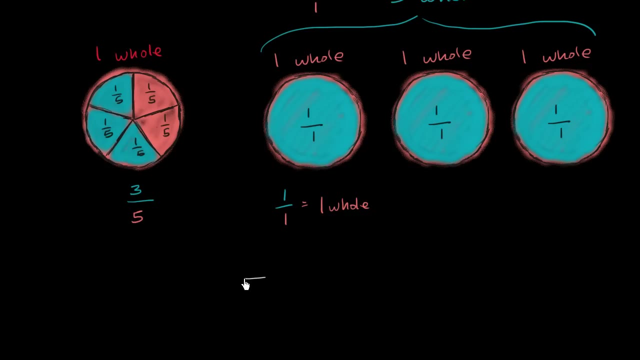 So this is equal to three wholes. So three over one is the same thing as the number three, And let me make sure, let me emphasize that, Let me draw this on a number line. So, once again, let me go all the way to three. 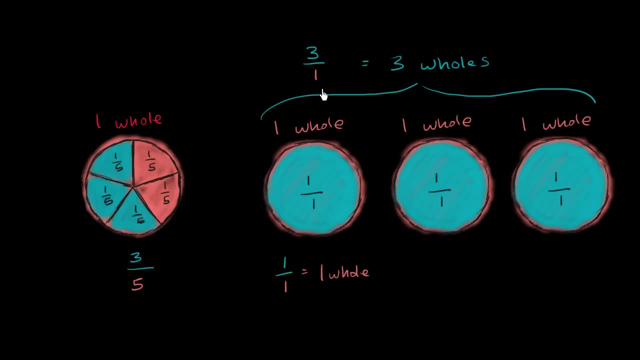 So I could call this 3: 1-ths. So this is interesting. Now we're seeing where the top number on a fraction is larger than the bottom one. But another way of thinking about this fraction symbol is that it's division. So you could view this as: 3 divided by 1 is equal to 3.. 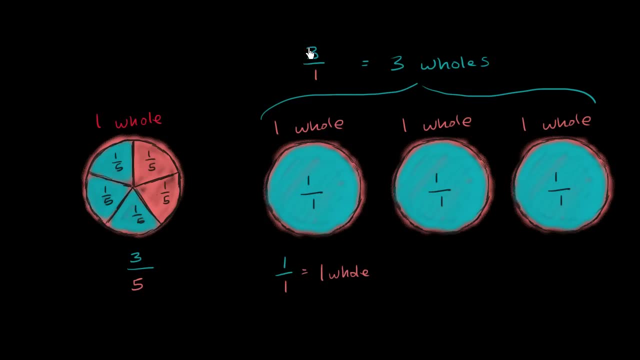 Or you could say: well, 1 over 1 is a whole, and I now have 3 of them, So this is equal to 3 wholes. So 3 over 1 is the same thing as the number 3.. And let me make sure, let me emphasize that.